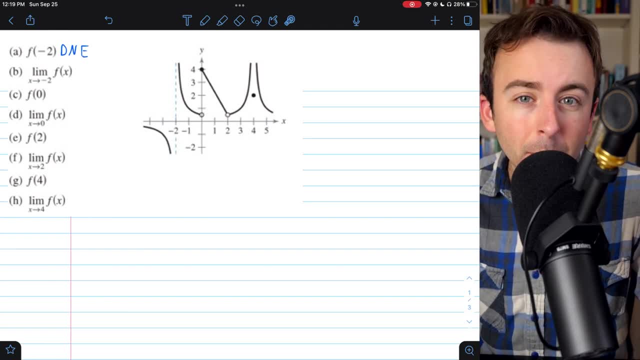 add no value at x equals negative two. But remember the function's value, whether defined or not at negative two, has nothing at all to do with the limit as x approaches negative two. Notice, in this limit no direction is indicated, whether we're approaching from the left or the right, So that means it's a two-sided limit. 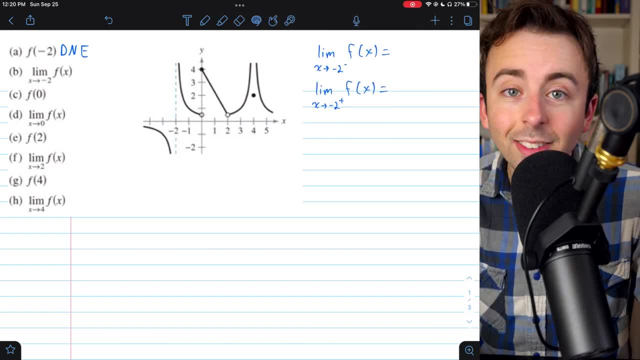 To evaluate a two-sided limit, we need to consider the one-sided limits. Let's begin here with the limit of our function. As x approaches negative two from the left, So here's: x equals negative two And this means that we're going to be approaching from the left, But remember, we're approaching on our function. So 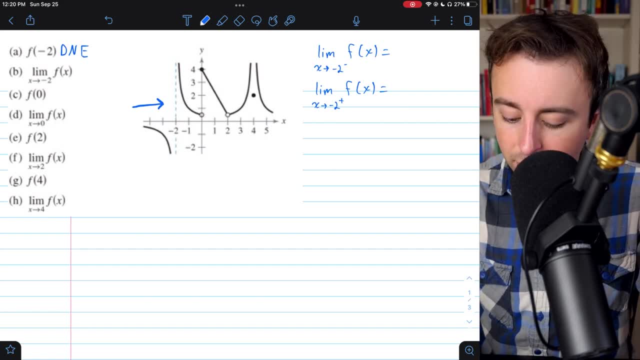 it's what the function is doing that is important to the limit. So we're staying to the left. of x equals negative two And we're looking at our function, which is right here. This is to the left of negative two on our function. What is our function doing as x approaches negative two? 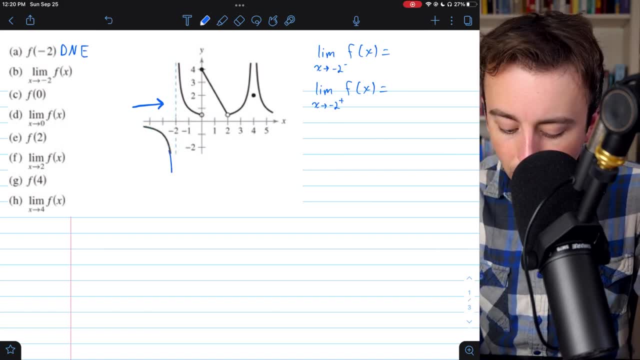 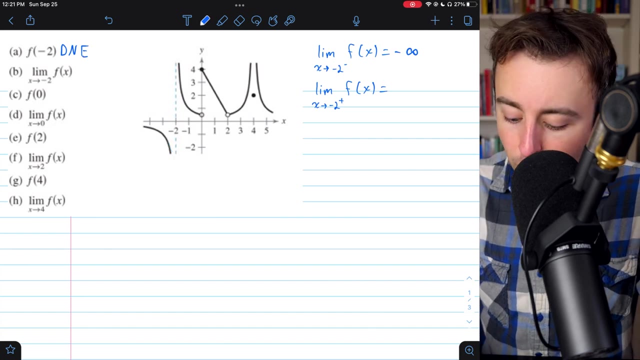 Well, we see that it's just going off downwards towards negative infinity. So our limit as x approaches negative two from the left of our function is negative infinity. The function is just getting very, very negative. Now. the other one-sided limit is the limit of the function as x. 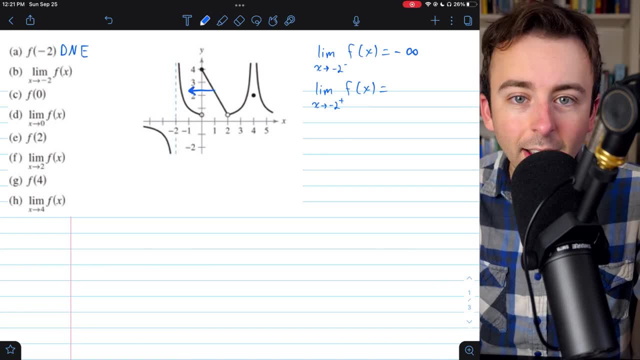 approaches negative two from the right. So we're over on this side, over here And again. remember we're staying on the function. We're wondering what does the function do as we approach the negative two x coordinate, And looking at this function as we approach x. 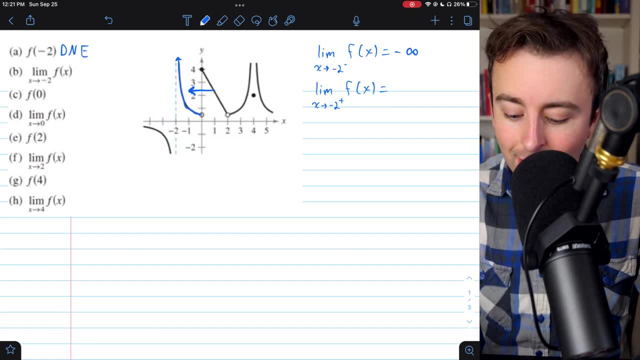 equals negative two. this function from the right is just veering off to positive infinity. So from the left we found it was going to negative infinity, But from the right we can see that it's going off to positive infinity. So that is our limit from the right. Now, since the one-sided 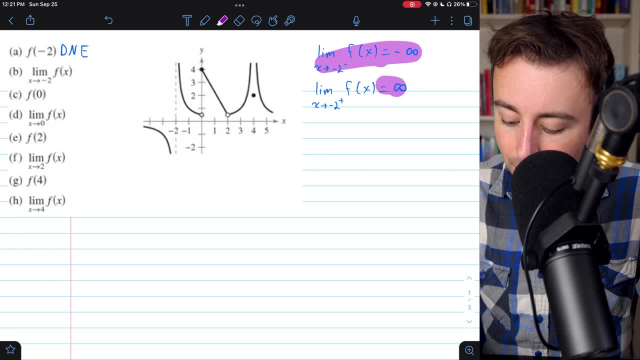 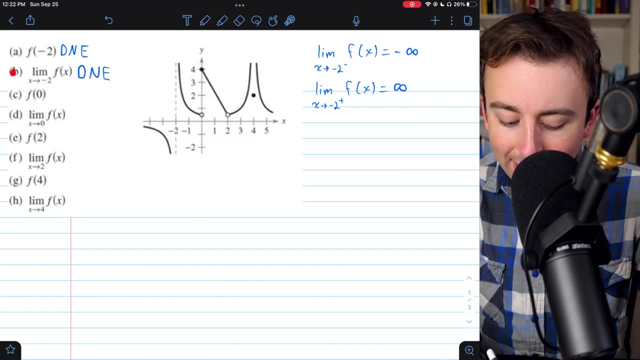 limits are not equal, this one's negative infinity, this one's positive infinity. So we're going to take the other one, the positive infinity, And then this one's positive infinity. Since they're not equal, the two-sided limit does not exist. Remember, that is the definition of a two-sided limit, not 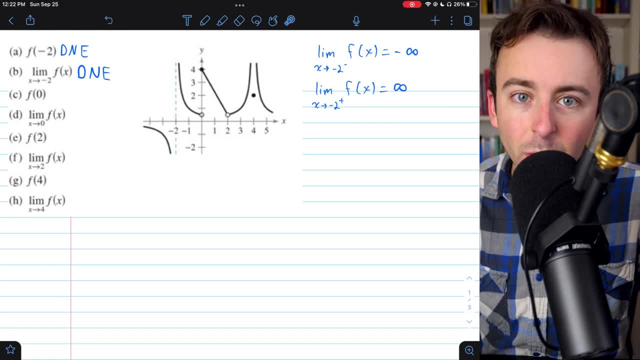 existing when the one-sided limits are not equal. All right, moving on to letter c, this just asks us to identify the function's value at x equals zero. So we come over to x equals zero. What is our function's value there? Well, it's not this right here which looks like it might be the. 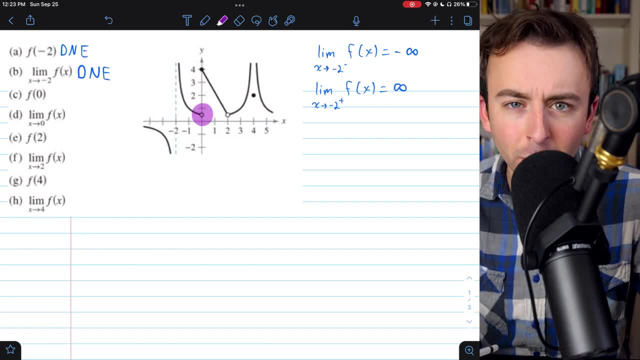 function's value. So we're going to take the function's value at x equals zero And we're going to one half. It's not that because that's an open circle, indicating the function does not take that value there. Instead, we want to look at the filled in circle saying, hey, this is the actual value of. 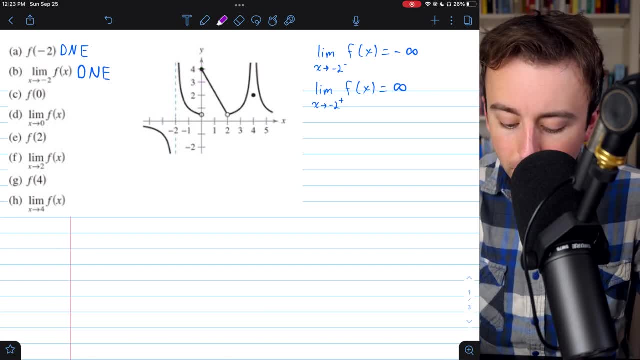 the function. at this point, When x is equal to zero, the function's actual value is four. So f of zero is four. Again, that's indicated to us by the filled in circle, in contrast to the open circle where there is a little hole, or what we might call actually a jump, because our function 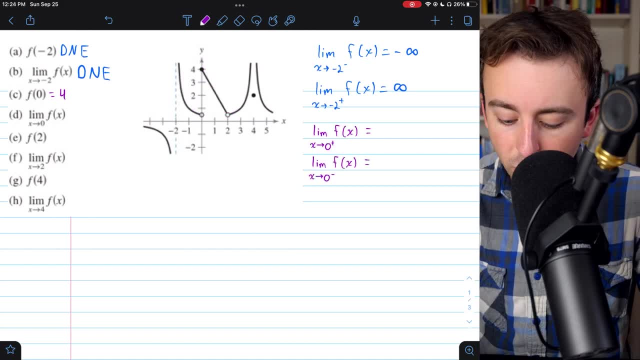 jumps from down here to up there. Now on to the limit of our function as x approaches zero. Again, this is a two-sided limit, So to evaluate it we need to consider the one-sided limits. Let's begin with this one: the limit of our function as x approaches zero from the right. So here's: x equals. 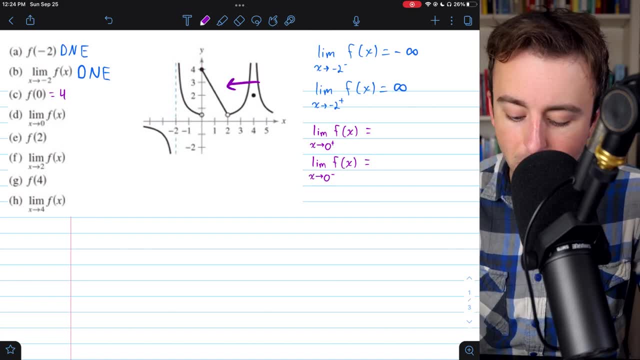 zero. We're going to be approaching from the right And we're staying on our function. What is our function doing as we approach? x equals zero from the right. Well, it looks like our function is getting closer and closer to four Again, that's. 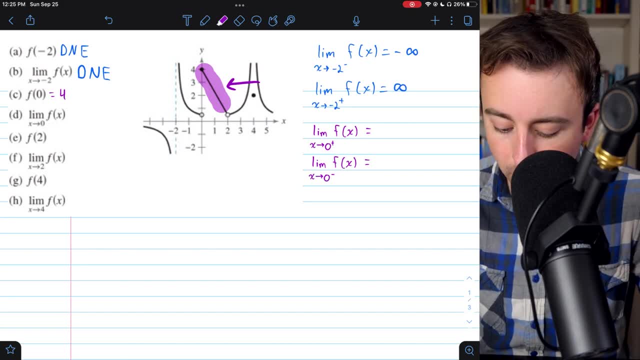 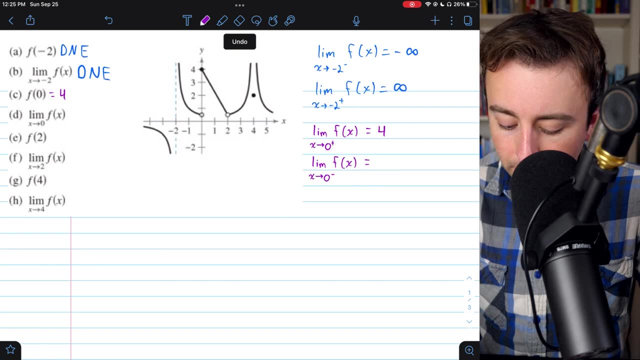 from the right. That's what's happening as we go towards. x equals zero, The function is approaching a value of four, And so that is the limit from the right Now, the limit of our function. as x approaches zero from the left, we're coming in hot from this direction. We got to stay on our 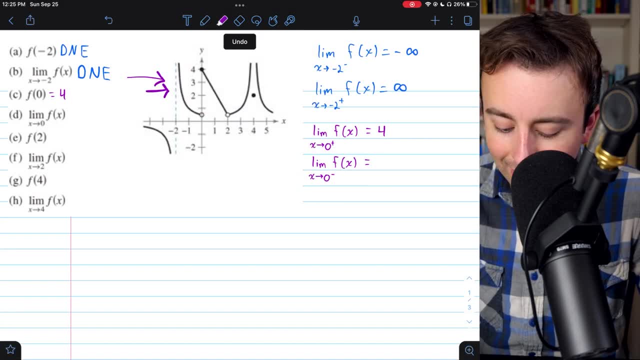 function. What's happening from the left? Well, from the left, our function is going down and down and it's approaching a value of what looks to be one half. That's the limit from the left. Again, here we see that the one-sided limits are not equal. From one direction we're going towards. 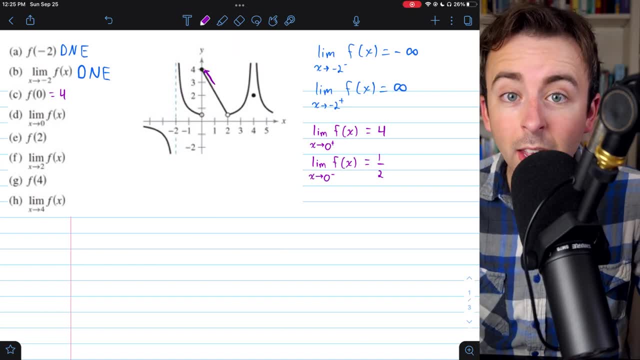 a half. From the other direction, we are going towards four. Again. the actual value at x equals zero, which we know is four. does not matter for the limit. As we approach from different directions, the limits are different, Thus the two-sided limit. 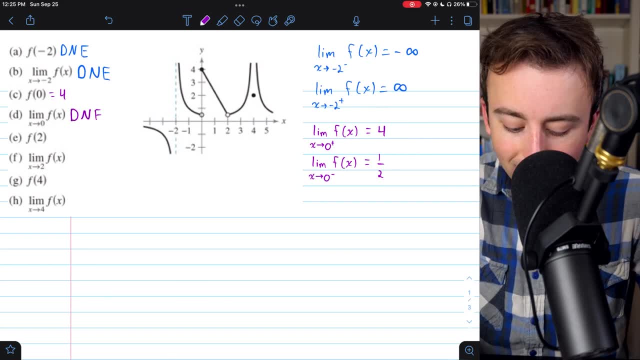 again in this case does not exist because the one-sided limits are not equal. Next letter e asks us the value of our function at x equals two. So we come over to the graph and look at this vertical line where x is equal to two. What's the value of the function here? 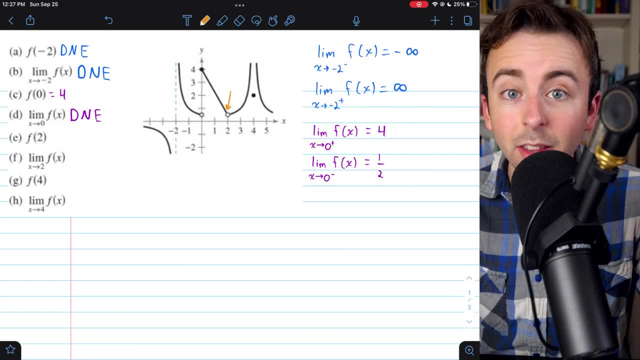 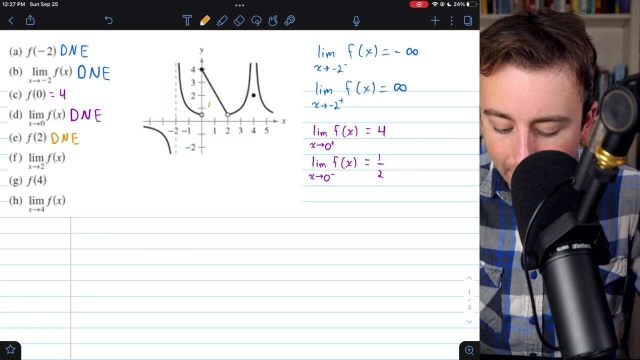 Well, we can see there's just an empty circle indicating that the function takes on no value at x equals two. So at x equals two, our function does not exist. Two is not in the function's domain. Remember, with x equals zero we also had this open circle, but we saw the function did. 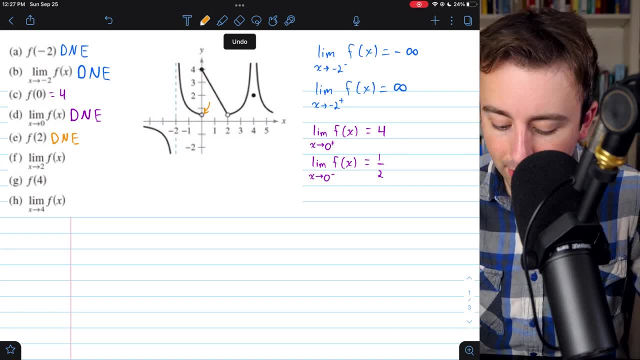 actually have a value with this filled-in dot. that was above it, But in this case, at x equals two, there is no filled-in dot, There's just the open circle. All right, let's then move on to the limit. So we're asked to find the limit of the function as x approaches the limit. 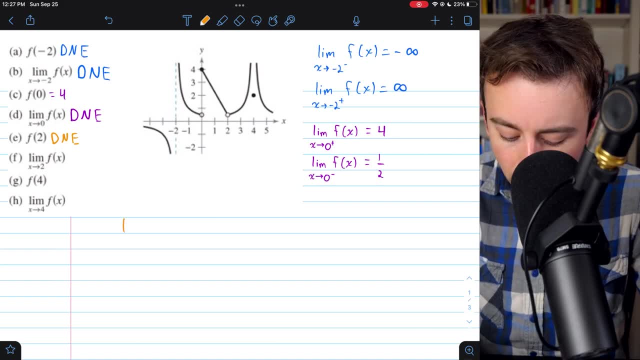 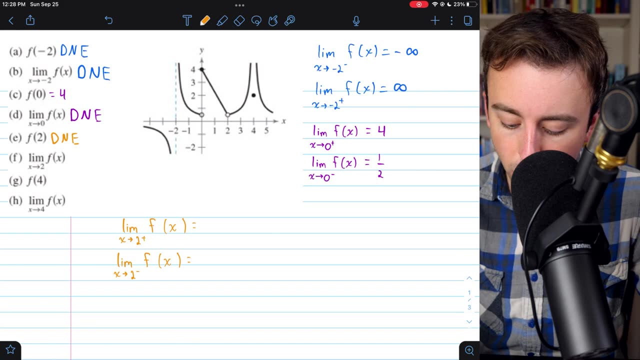 Again, to evaluate this two-sided limit, we will need to consider the one-sided limits. Let's begin with what our function is approaching as x approaches two from the right. So we're coming in from this direction, from the right of x equals two. And what is our function doing? 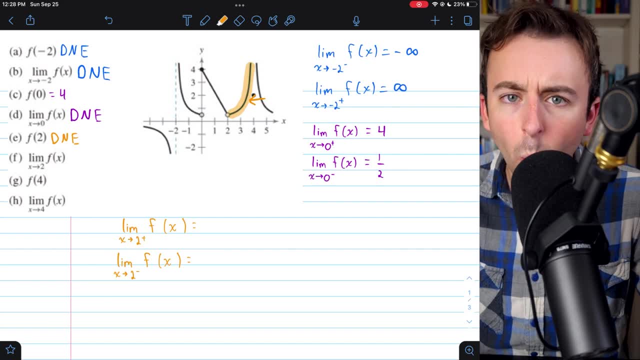 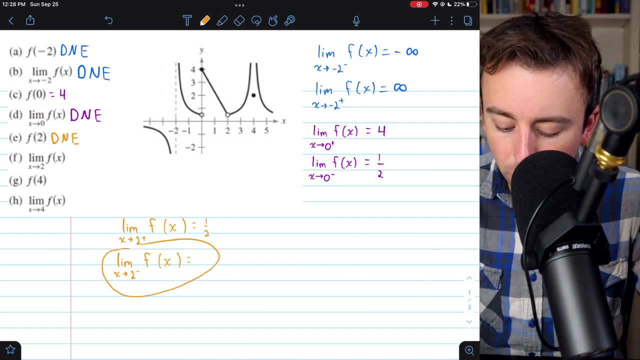 It's approaching that same value that we had before of one half. So the limit as x approaches two from the right is a half, And then the limit as x approaches two from the right is a half From the left. now we're approaching two from this direction, And what's our function? doing as 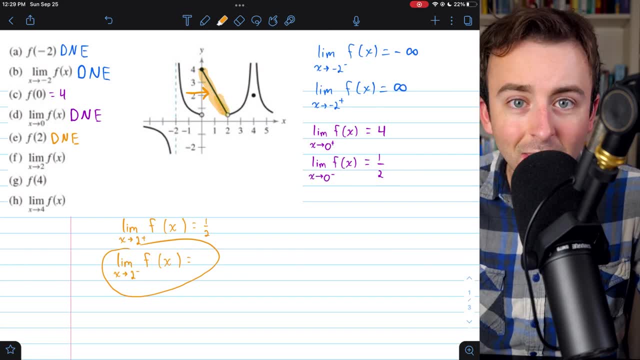 we approach two from the left, It looks like it's doing the same thing. From the left, it's also approaching one half. So the limit from the left is a half. So what we see here, even though the function doesn't have a value at x equals two, its limits from both sides are equal. They're both a. 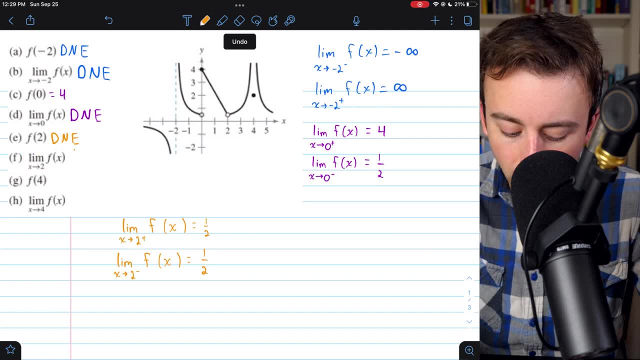 half, So the two-sided limit is also a half. So we're approaching two from this direction And one more, x coordinate. we're going to look at What's the value of the function at x equals four. Well, come over to where x equals four And we see that indeed we have a point on our function. 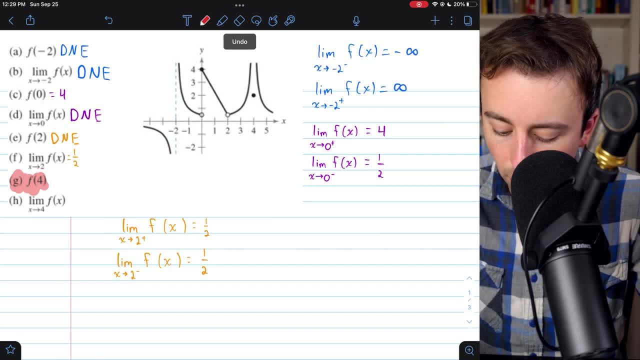 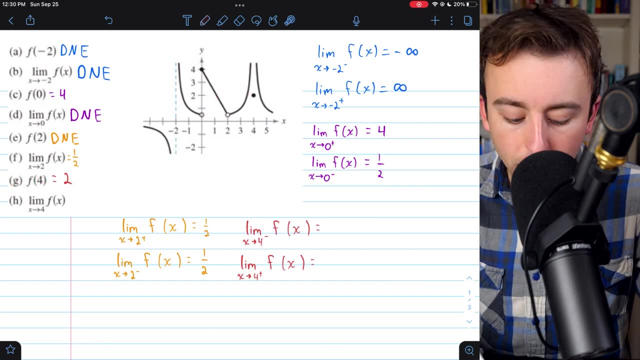 here It's this filled in: dot. At x equals four, the value of our function looks to be two, So f of four is equal to two. Now to evaluate the two-sided limit as x approaches four, we will look at the one-sided limit. 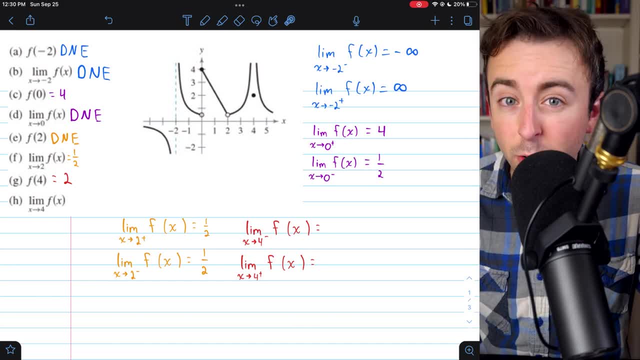 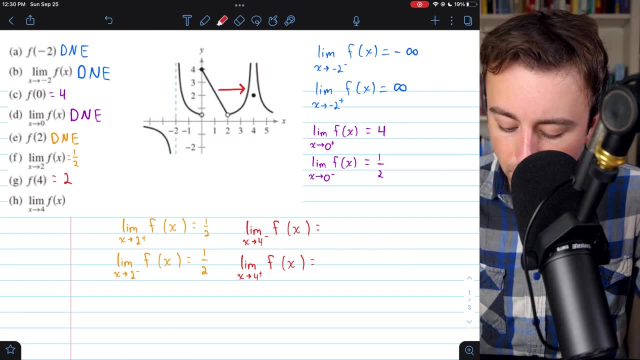 The limit of our function. as x approaches four, let's do from the left first, just to switch it up. We're approaching four from the left, So we're coming in from this direction. What's our function doing? Well, as we're approaching four from the left, looks like the function is just veering off. 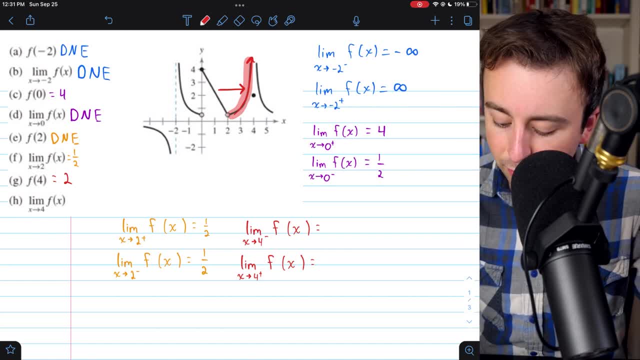 to positive infinity. So that is the limit from the left, The function is going to positive infinity. Then what's the limit of our function? as x approaches four from the right, We're coming in from this direction, We're approaching on the function approaching four from the right, and it looks like the function is just. 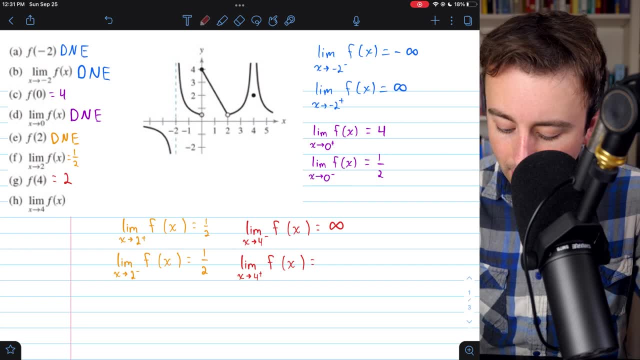 veering off again to positive infinity. So here the one-sided limits: they're both infinite, but they are both equal in this case. So we can say that the two-sided limit, as x approaches four, is positive infinity. So notice, through all of these examples, we have points where the function's value 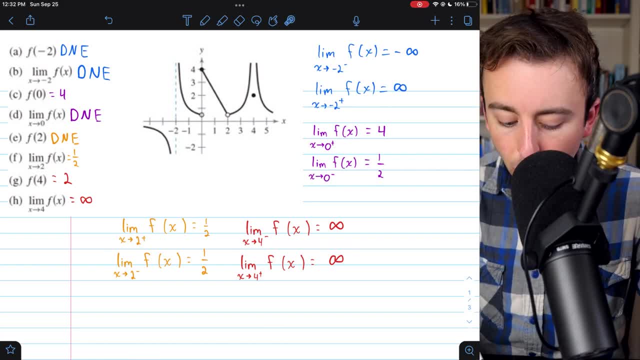 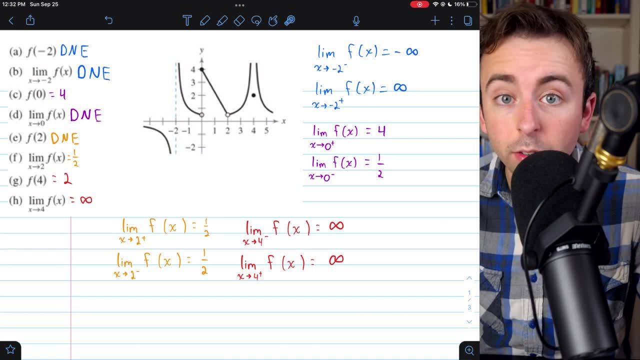 and the limit both don't exist. We have an example where only the four-sided limit is equal to the function's value exists, but the limit doesn't. We have an example where the limit exists, but the function's value doesn't, And we have an example where they both exist, even though in this case, 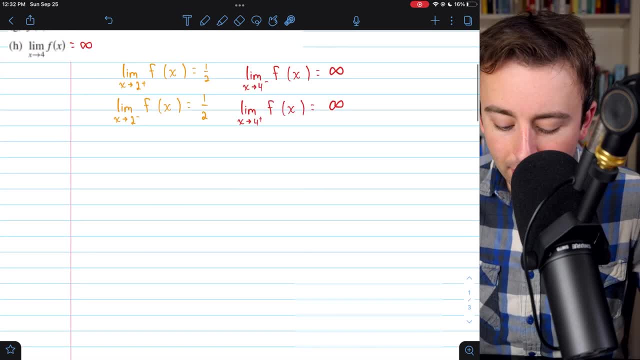 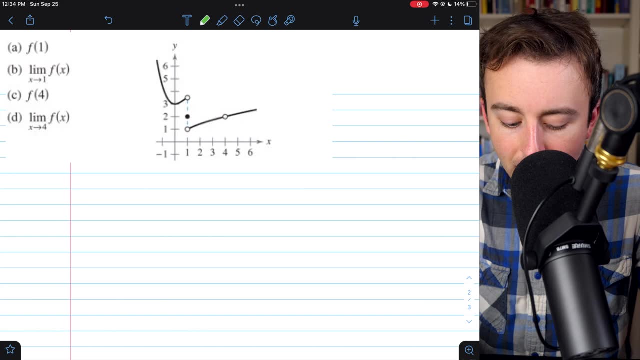 the limit happens to be infinite. That's still a limit. So give this example a try yourself. Four questions, Hopefully you can do it All right, I'll go over these real quick. The value of the function at x equals one we see here at x equals one. the filled-in circle tells us our 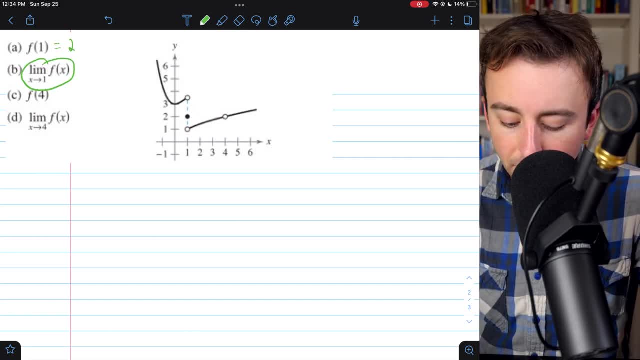 function has a value of two. Now the limit of the function at x equals one. we see here, at x equals four. we see that the value of the function as x approaches one does not exist, because as we approach from the left it looks like the function's going to three and a half. As we approach from the 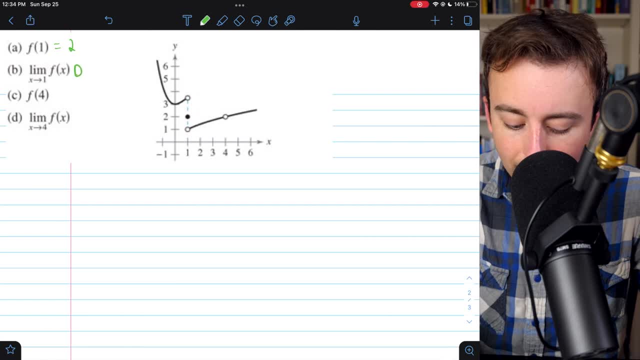 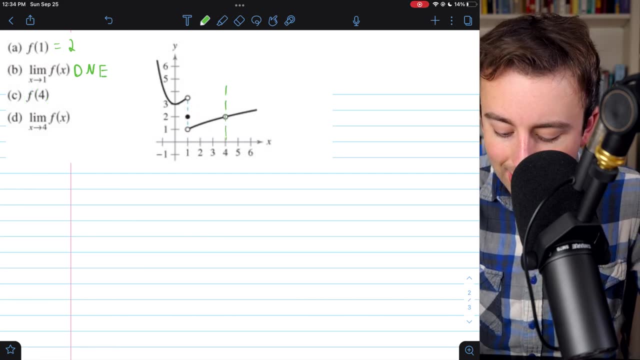 right, it looks like the function is going to one. So the two-sided limit as x approaches one doesn't exist. The value of the function at x equals four. we see that doesn't exist because all we've got is an open hole. So f of four does not exist, But the limit of the function as x.